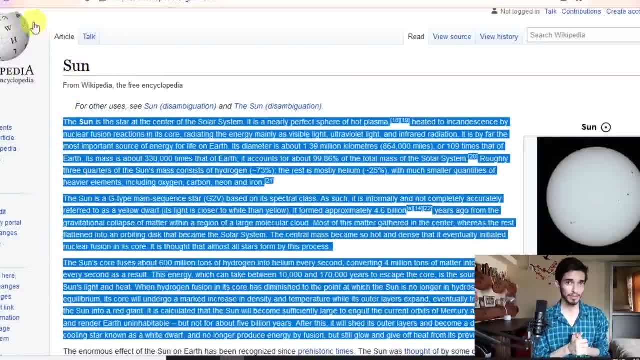 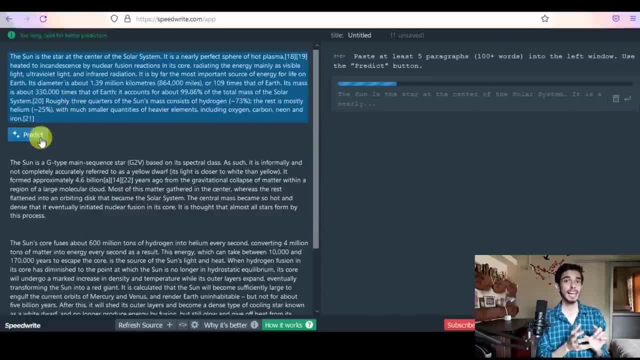 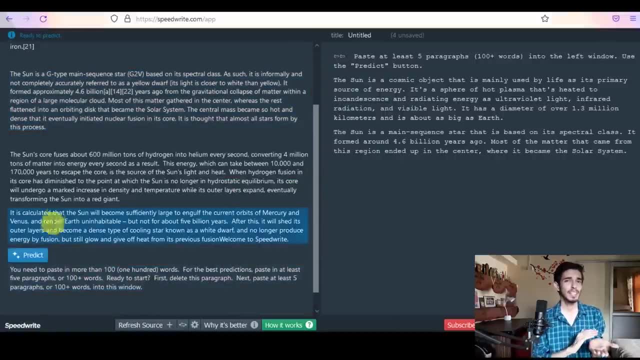 Sun, But I can't just copy and paste it from Wikipedia, So what I can do is this: I can copy this to SpeedWrite, And there SpeedWrite uses an AI to rewrite the text given to it in a completely unique way, And every time you do it it will generate a completely new. 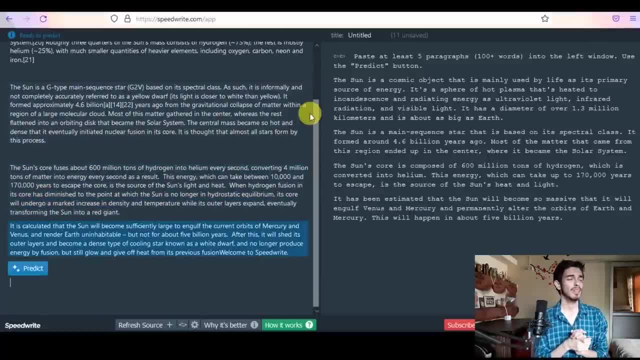 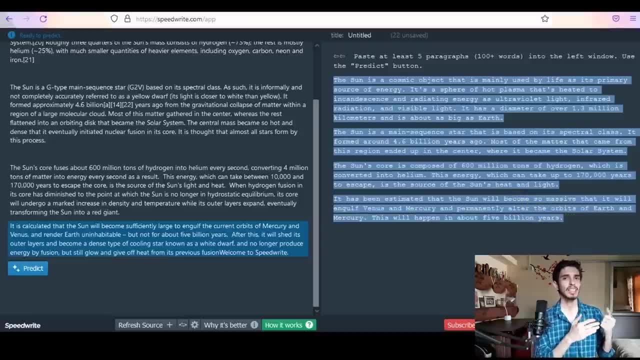 text. So, if wisely used, this tool can help you save a lot of your time, which you can use to do something better than those useless and redundant assignments. So now let's come back to Kung Fu Mathematics. Why I call it Kung Fu Mathematics is because the 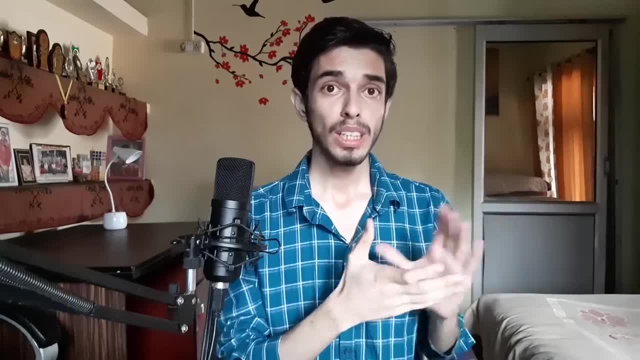 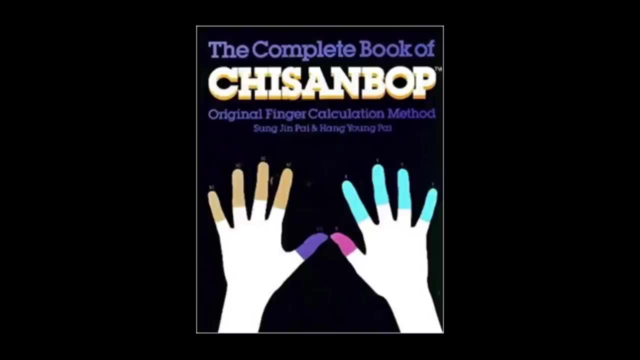 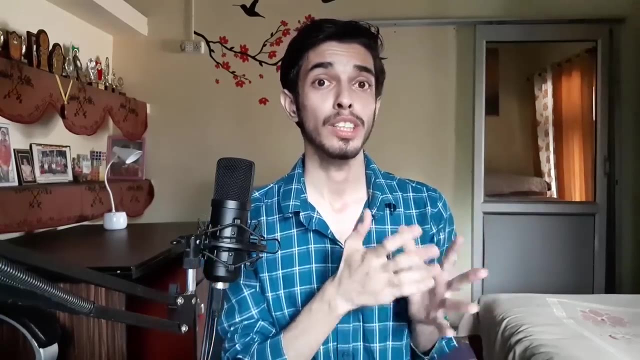 students doing. it looks like they are doing Kung Fu, But originally this method is known as Cheesan Bob, And the book that I am using to teach you this method is The Complete Book of Cheesan Bob by Yung Pai. It uses our fingers in a really efficient way and with which we can do phenomenally. 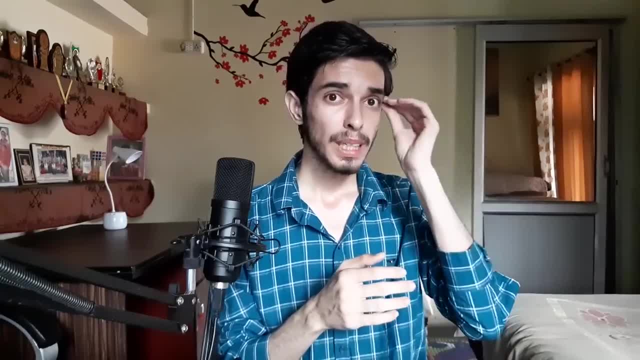 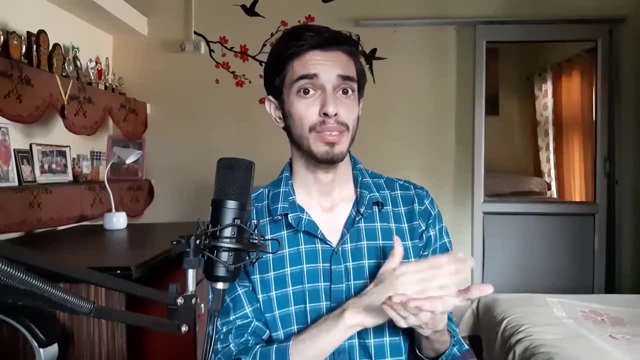 fast calculations, So let's start with Cheesan Bob. It uses our fingers in a really efficient way and because in this method our brain rests, Our brain has only one job and that is to count, nothing else. In other methods, like in Left to Right and other methods, 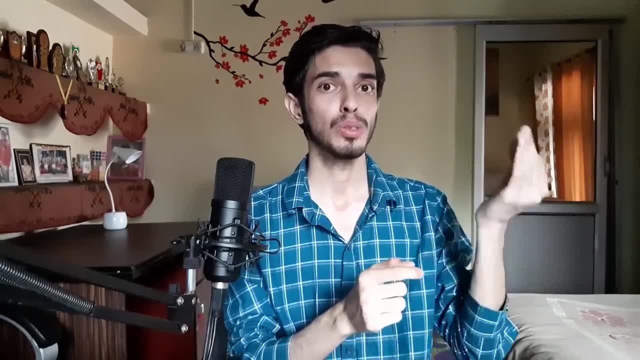 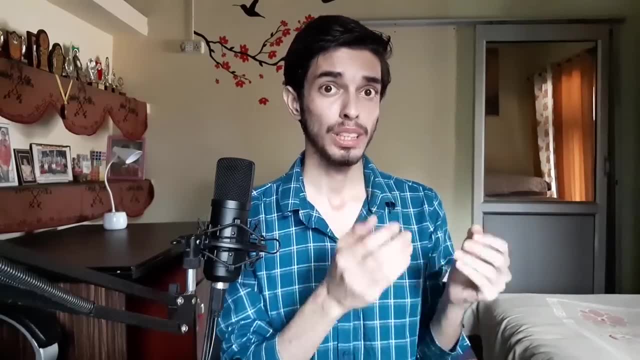 we always needed to keep track of the answer. We needed to use your memory. Our brain was stressing a lot, but in this method our brain is mostly relaxing and our fingers are doing most of the work. So the most crucial part of this method is: 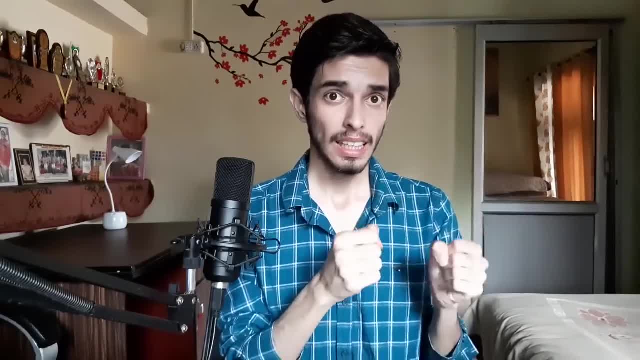 being able to represent numbers on your hands. I am using just my fingers in this method. It contains much faster numbers and you can process numbers really fast using it. The Hilbert method actually完 total Connected. était гл��'€€ std ShapeXh 안이�унк에. 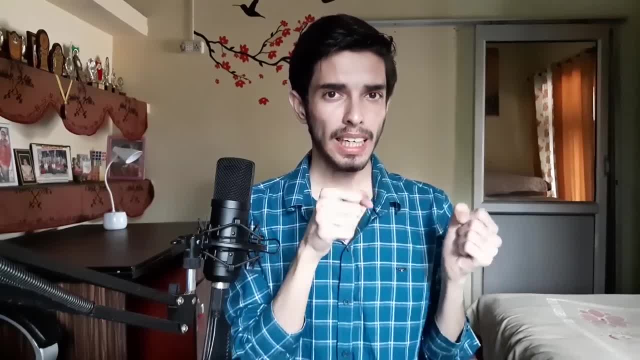 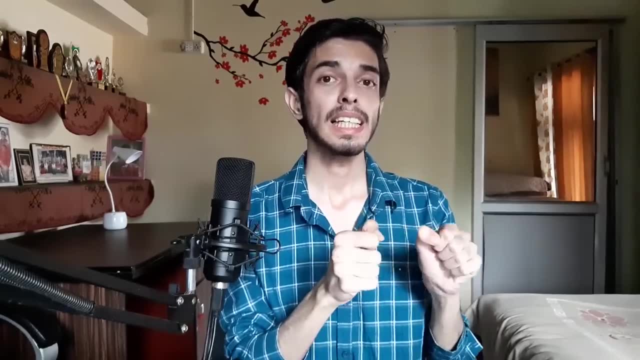 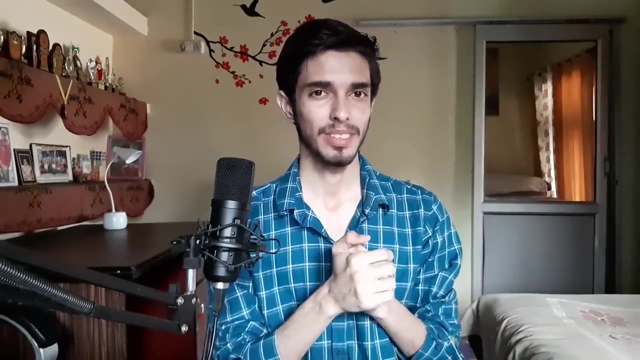 Spec effects. But the faster you can switch from one number to another number- and there are some rules- the faster you can apply those rules, the faster you will calculate. so this one will take a little bit of practice, but after practicing you can do phenomenally fast. calculation really is the end. it is not that tough. so now at 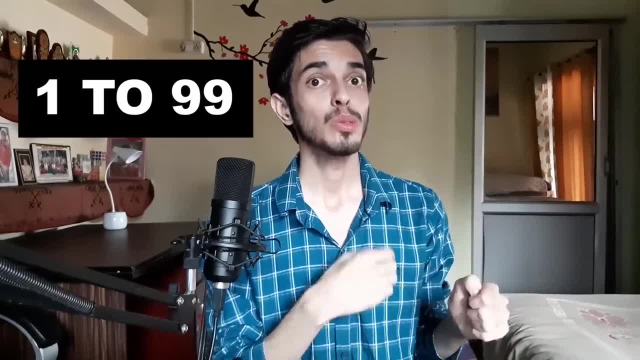 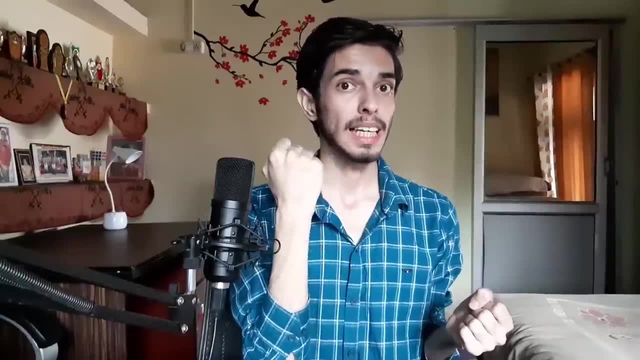 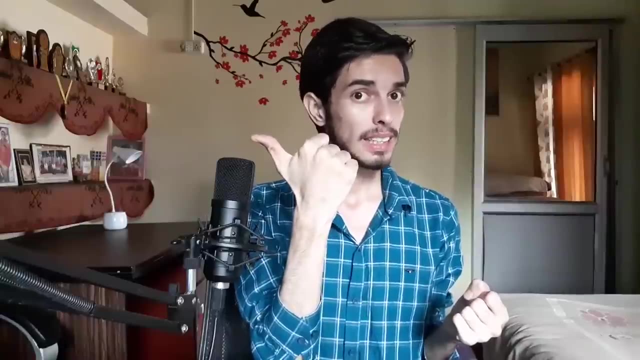 first, let's learn how to represent numbers from 1 to 99 on your hands. our right hand represents numbers from 1 to 9. it is like this: so this is one, this is two, this is three, this is four, simple, but now this, not five. this is five, okay, this is five. and this is six, this is seven, this is. 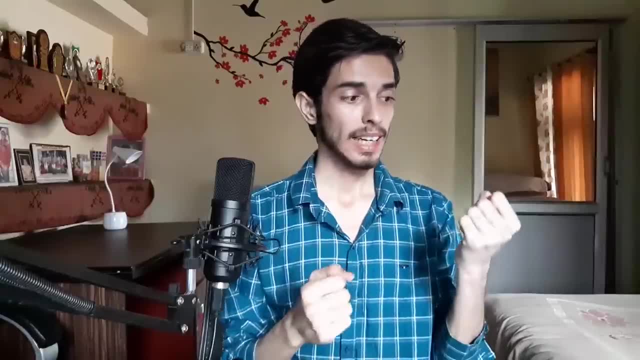 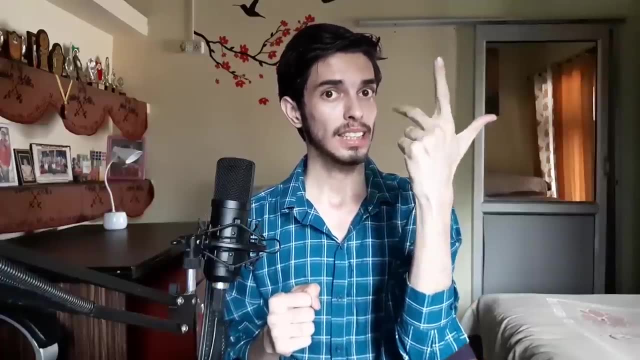 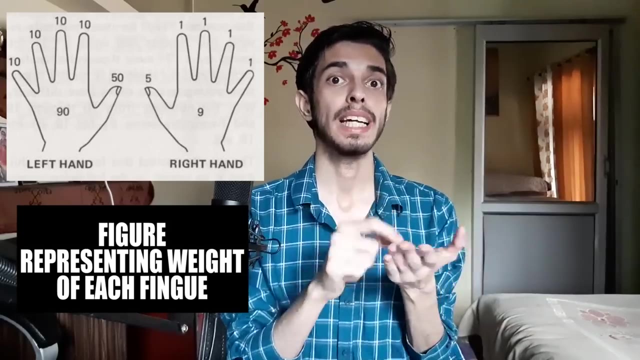 eight and this is nine. so from one to nine in here, and this is 10, 20, 30, 40 and this is 50, 60, 70, 80 and 90.. now we have the representation. now we can represent any number from 1 to 99 on our hands. So let's take an example. Let us represent 12 on our hand. 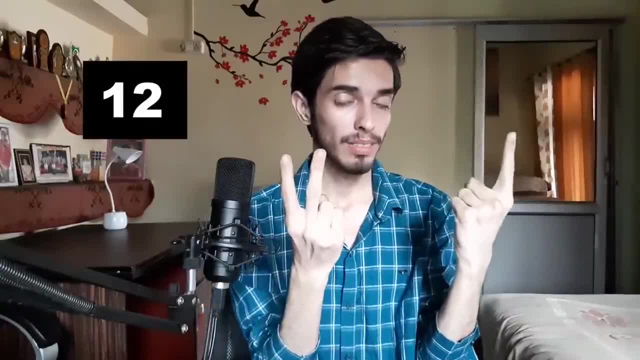 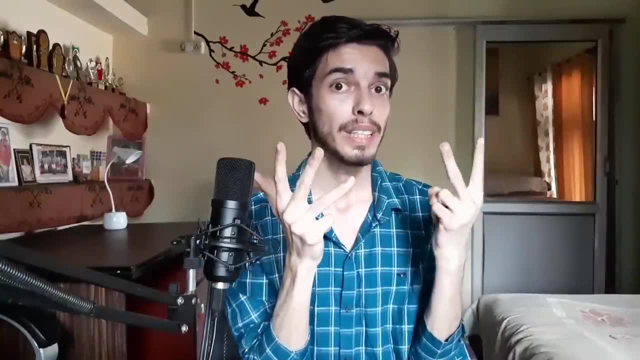 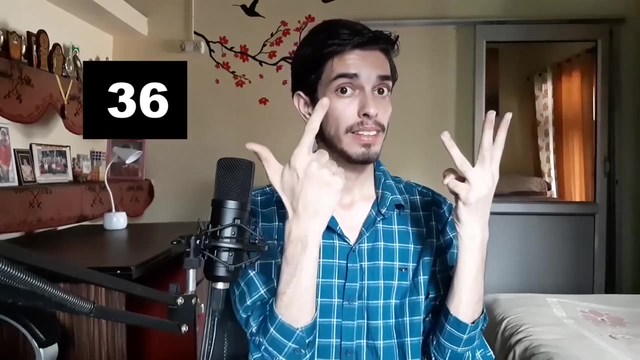 So see, this is 10 and we need 2.. This is 12.. Now let us represent 28.. So 20 and 5,, 6,, 7,, 8.. This is 28.. So now try representing 36 on your hand. So this is 10, 20,, 30 and 6,, 5 and 6.. So. 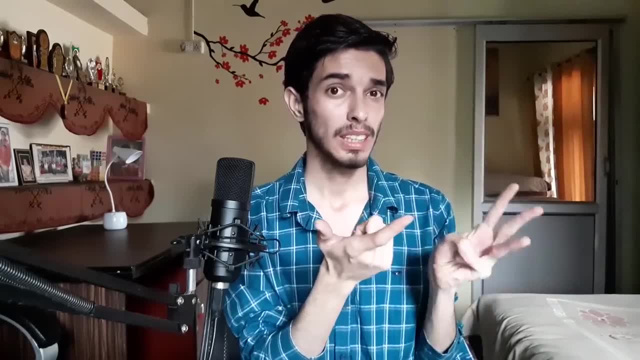 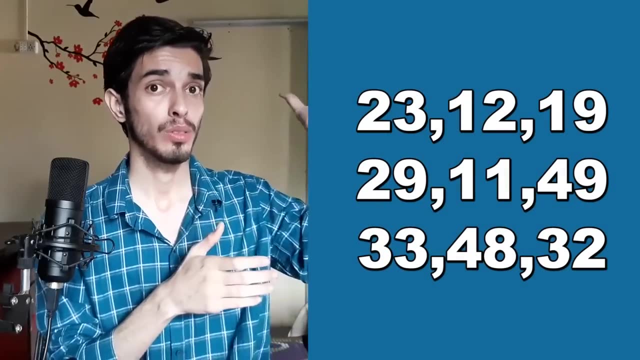 this is 36.. Now, this looks pretty simple. How simple is this? But this is really, really powerful. Now try to represent these numbers quickly on your hand, as fast as you can switch from one number to another number. Now, what you have learned is the essence of Chisholm, Bob or. 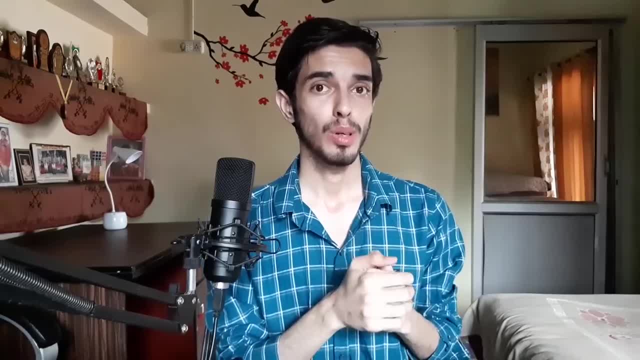 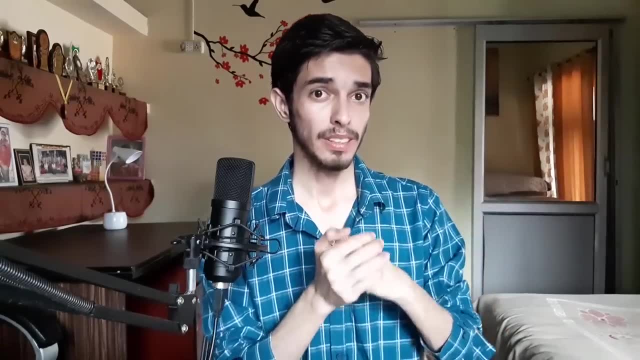 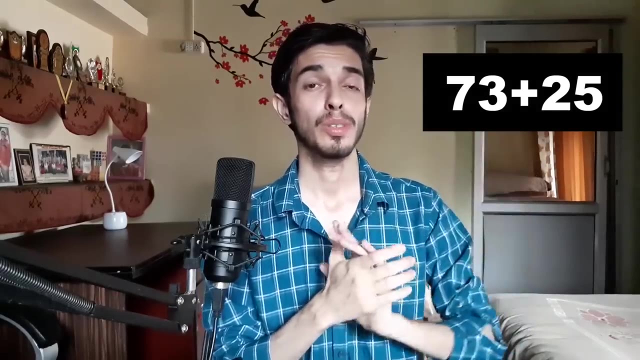 Kung Fu Mathematics. Now, with this, you can do any addition problem whose answer is less than 99 on your hands, using Chisholm Bob. So let us take an example: We need to add 73 and 25.. Now, firstly, you can also use left to right method, and this is a really easy problem, if you have seen. 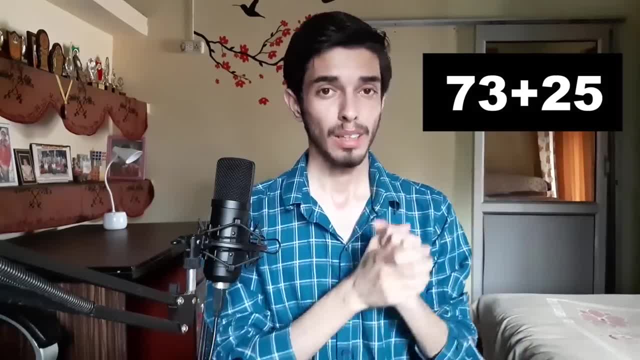 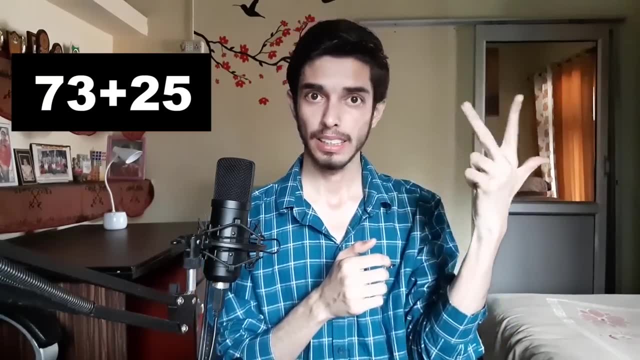 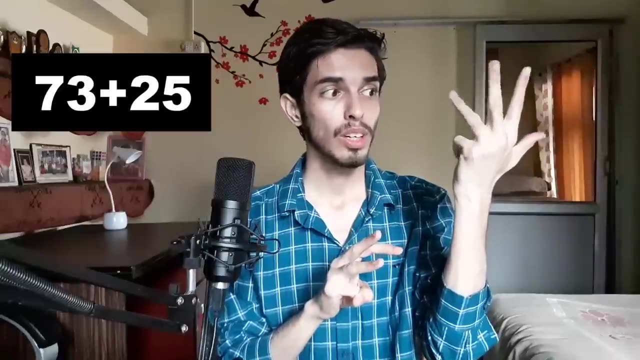 my previous all videos. There are tons of ways you can do it, But now we will use our fingers to do it. So first represent 73. How, 50,, 60,, 70. Now 3, 73.. Now represent 25.. So we have 20 in here. So 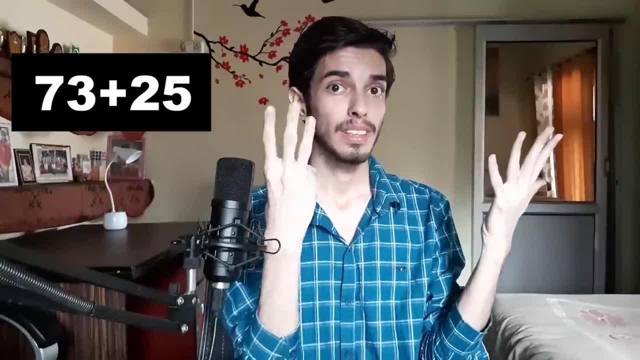 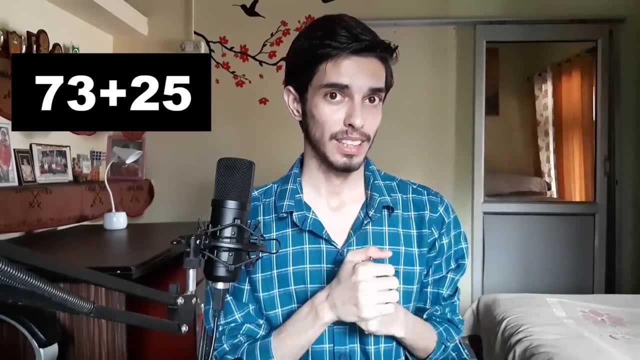 10,, 20,, 20 and 5, 5.. So what is this? This whole is 90 and this is 5,, 6,, 7, 8.. 98 is our answer. So right now I was explaining this, But in reality, if you do it, 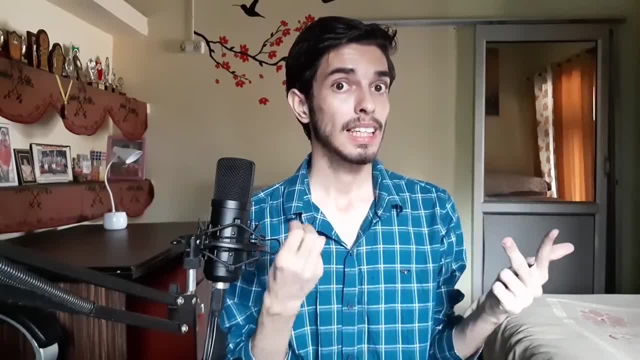 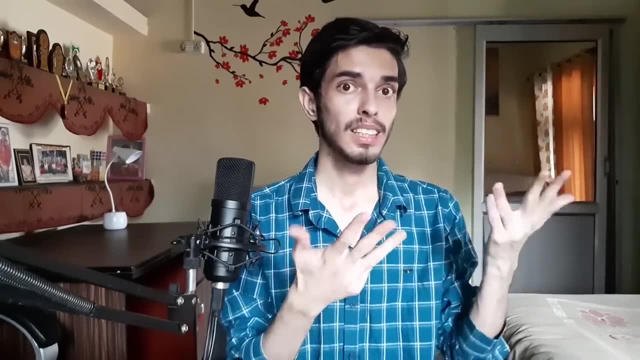 you just need to hear someone saying like 70, 3 and add 20, 5 and at the end count This is 90, this is 5, 6, 7, 8. So 98.. So in here our mind is resting. You can see it by using the left to. 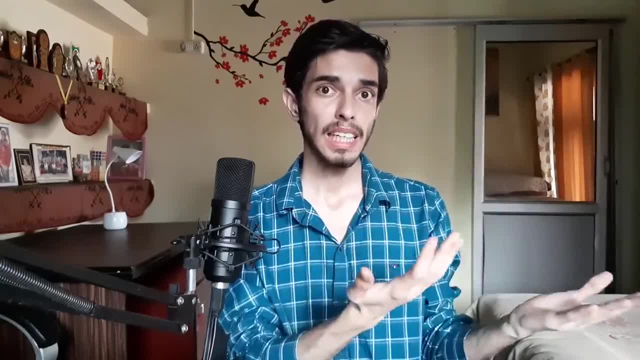 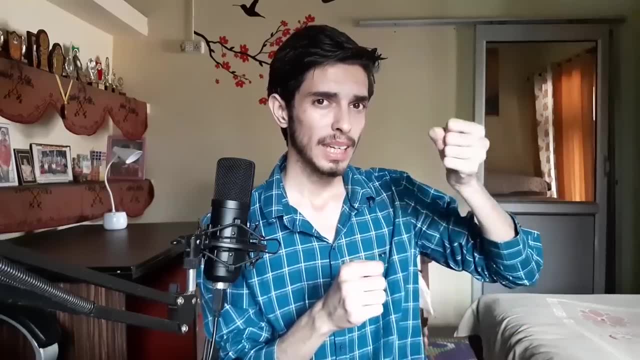 right method. There our mind is doing all the work, But in here our hands are doing the most of work. They are able to add long strings of numbers Because every time they add it they don't need to keep track of the answer. Their hands have the answer And in that answer they are adding further. 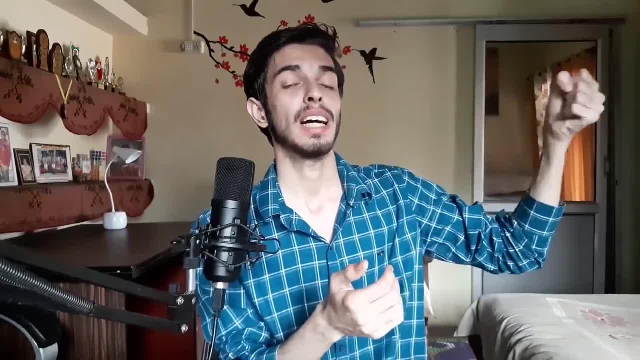 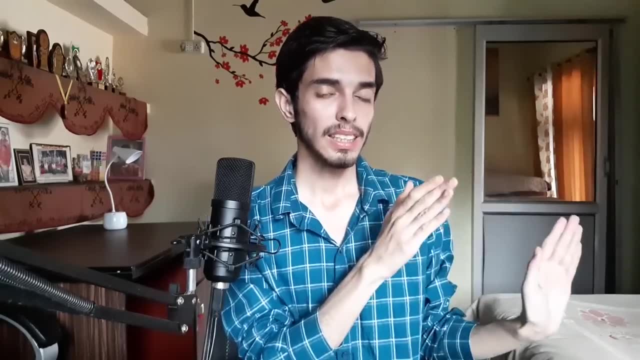 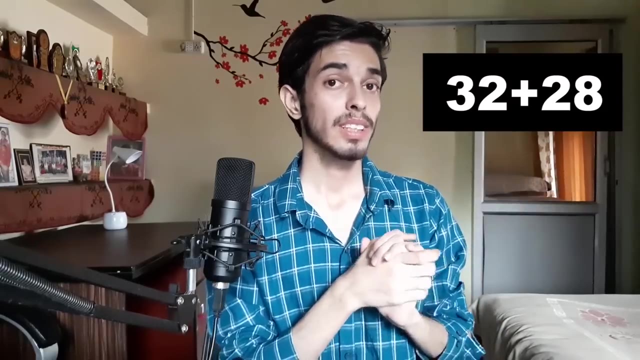 and then further, And by doing this they are doing that fast calculation. So now there is a little limitation in our hands. The previous question that I have taken is specially designed not to include that limitation. But let us take this question, 32 plus 28.. So let's first represent 32.. 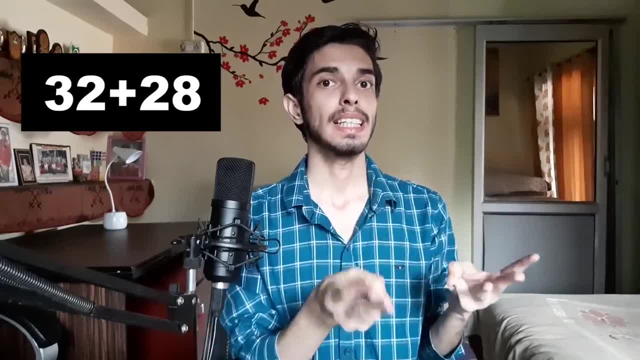 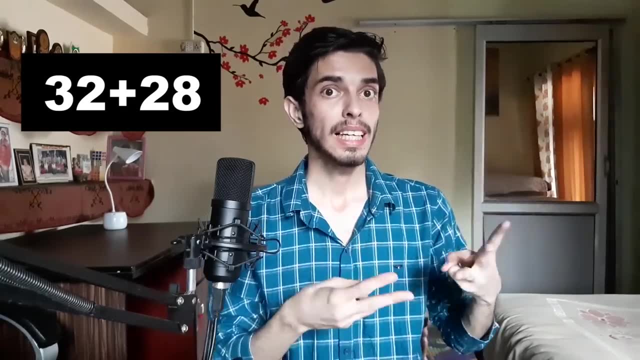 And 2. 32.. Now we need to add 28 to it. Now how would we do it? See, in here I have just 10.. So there is no 20 in here. Then what would I do? In here, you need to be creative with cheese and 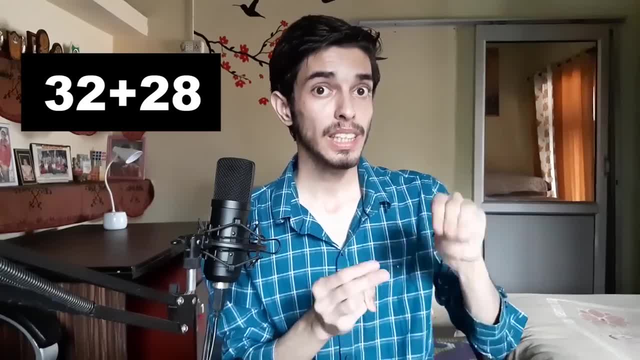 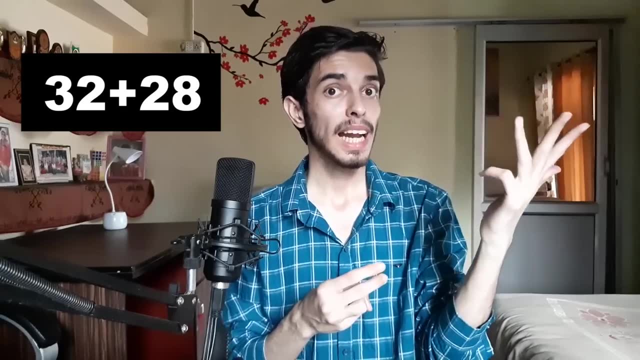 bob, By practice this will come automatic. So in here we need to add 20.. We don't have fingers for 20.. What can we do is this: We can add 50 and subtract 30. So we have 50. So see 30 plus 20. 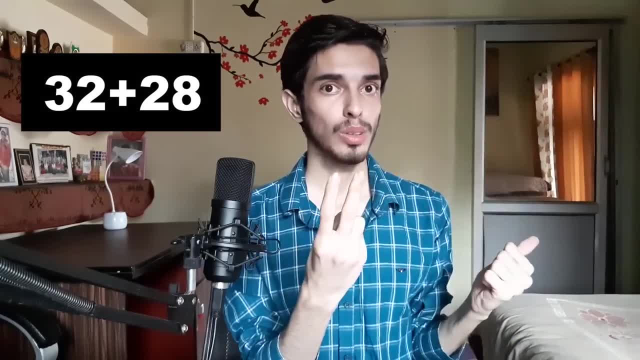 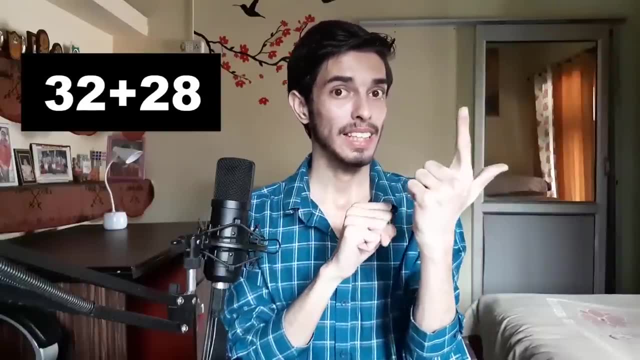 is 50. Now 28.. For 8: we also don't have fingers, So what we can do is this: We can add 10 and subtract 2.. So what we have in here, 50,, 60. 60 is our answer. So in cheese and bob, because we have 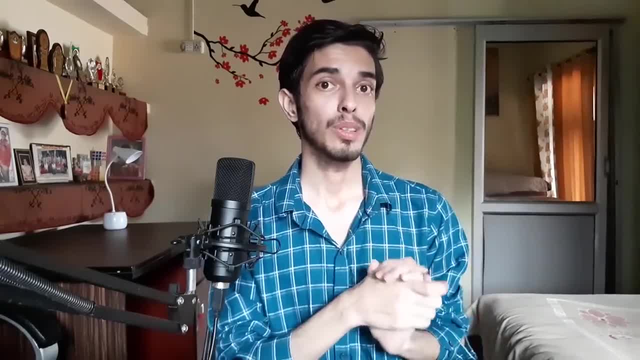 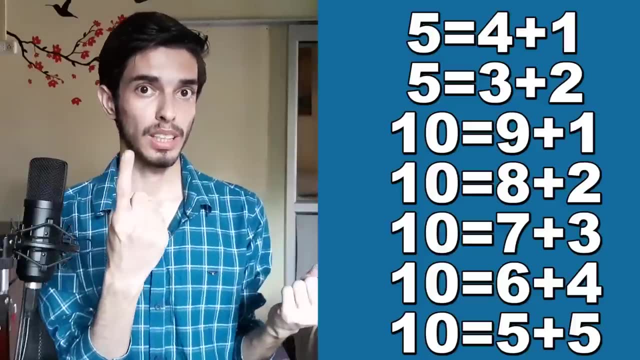 only 10 fingers. we have this limitation, which we can overcome by knowing these simple rules. These are like really simple rules, Like you don't need to memorize them. For example, let's say you have this finger opened already And now you want to represent 9 in here. How would you? 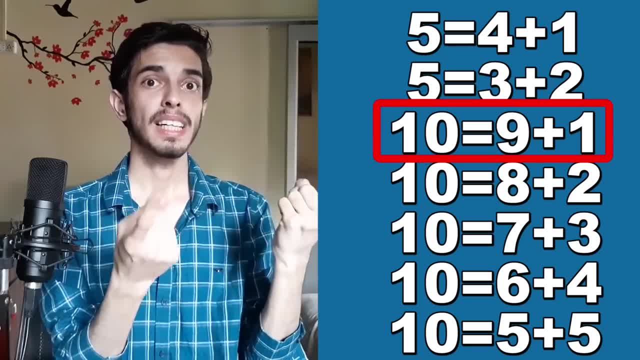 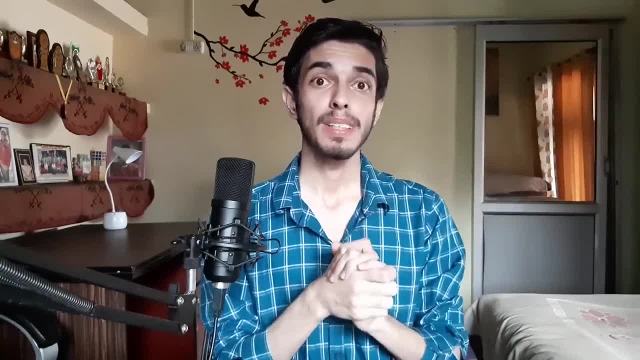 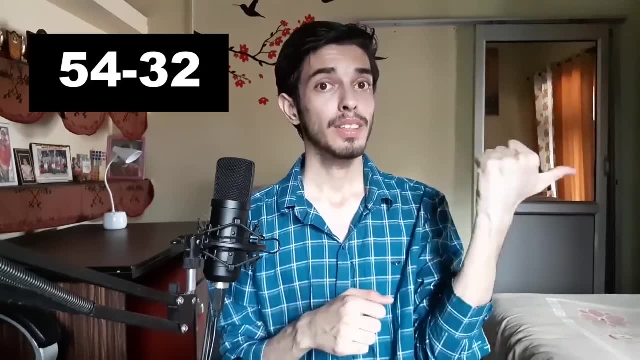 do it? It's simple, using this equation: Add 10 and subtract 1. The only thing that you need is the practice on your hands to do it even faster. Now let's take a subtraction problem with cheese and bob: 54 minus 32.. Try to do it yourself. How would we do this? See 54.. Okay, 54 minus 32.. Now in here. 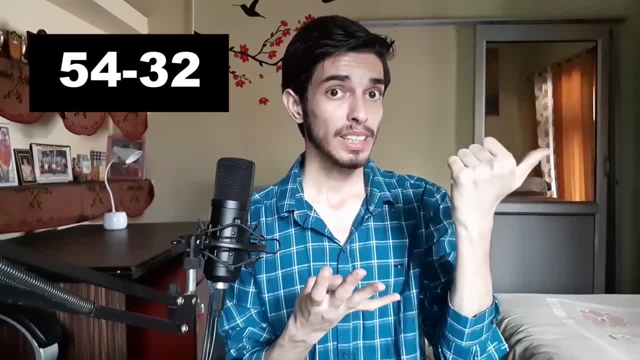 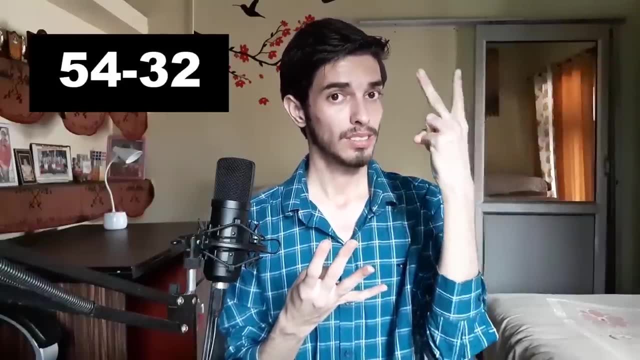 what we have this: We need to subtract 30 first. So what we can do is this: We can first subtract 2 and then add 20.. So this should be very quick: 20 and 2. We need to subtract 2.. What we have in: 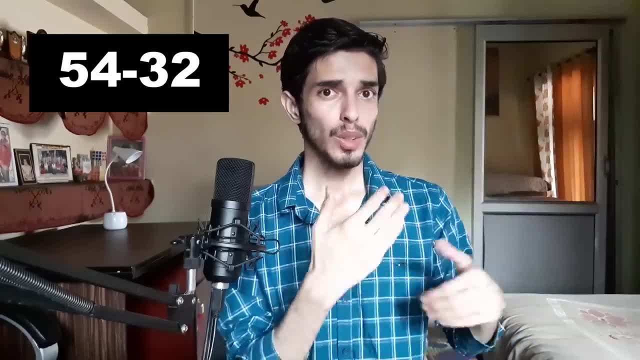 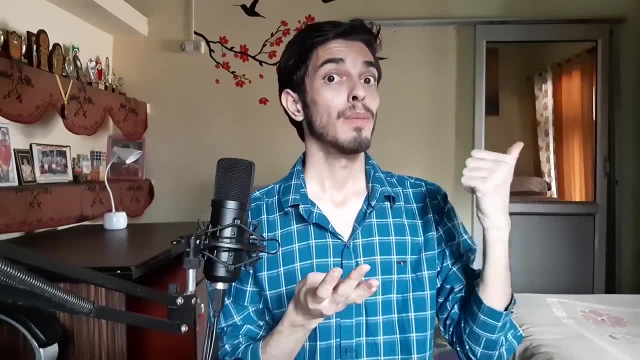 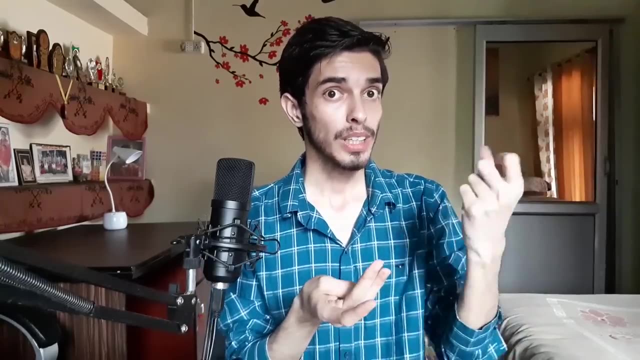 here 22.. So this is how easy cheese and bob is. So in reality, this should be this quick. Like someone saying to you You need to do this. He's saying 54 minus. He said minus 10.. Like, prepare your brain that he's saying minus. And he said 30. And quickly, 30 and 2.. We need to like. 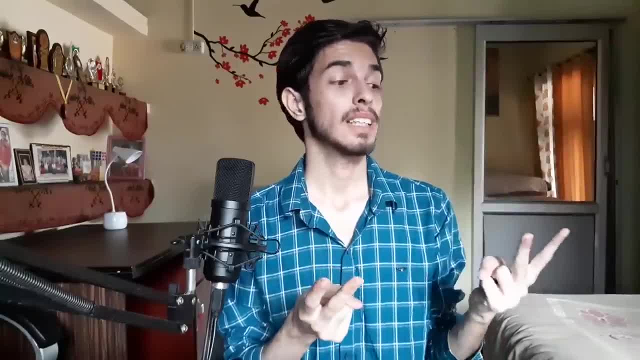 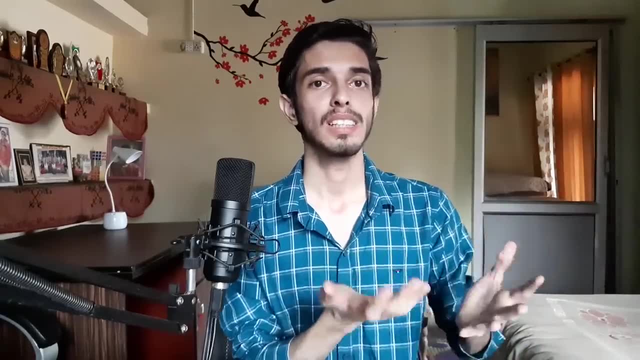 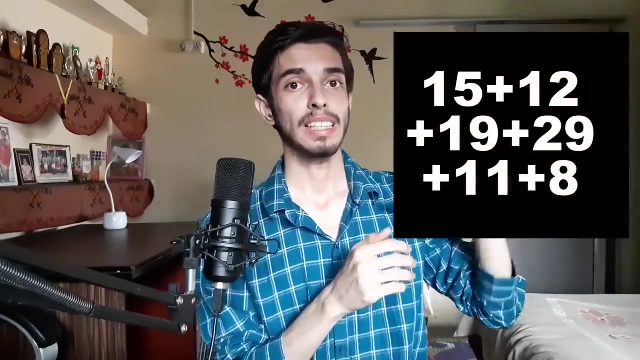 do not open it, Like subtraction is closing it. So what we have added? 22. Say it quickly, So like you have not taken any time to solve this problem. Your hands only just solved your problem. So this is basically the real power of cheese and bob. Okay, so now let's try this long addition problem. 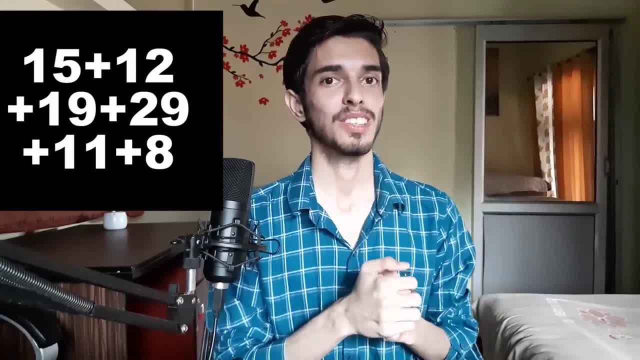 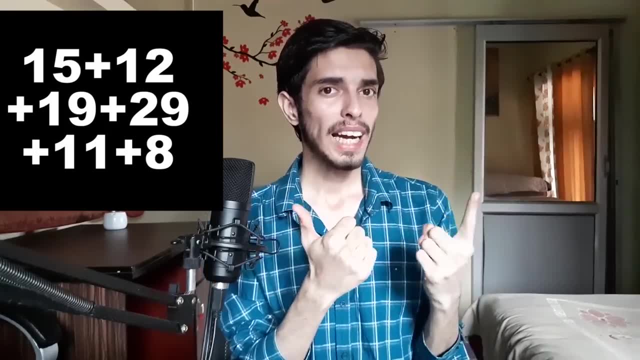 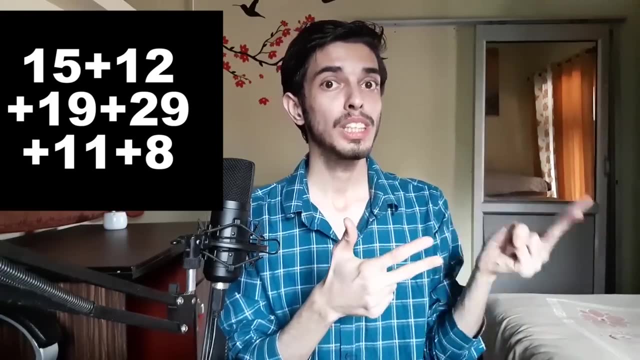 Like someone telling you 15 plus 12 plus 8 plus 29 and so on. How would you do it? So do it with mean: First represent 15.. So 15.. Now add 12 to it, So 12.. Now in here. this is the real thing. If you are doing it, otherwise, you would need to keep. 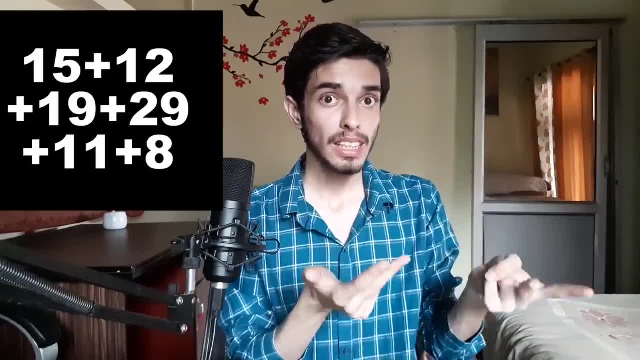 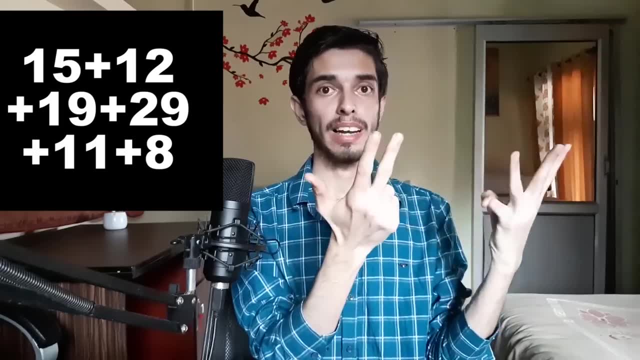 track of the answer, But now we don't need to keep track of the answer. Give us the next number in here. So now add 19.. So adding 10.. And now for 9. we don't have fingers, So what we can do is this: 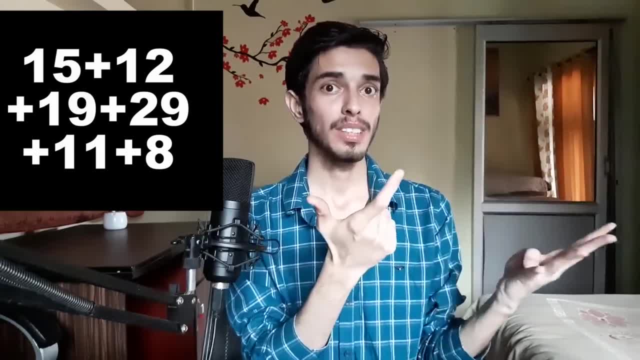 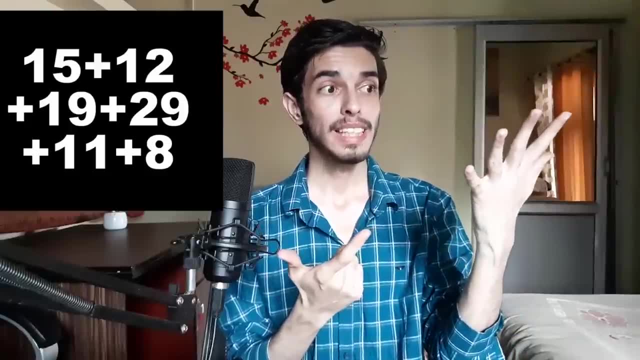 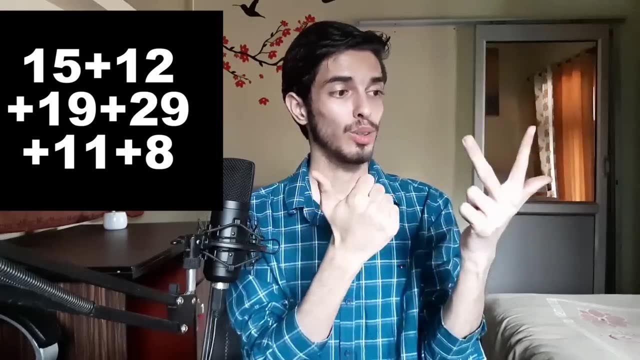 add 10 and subtract 1.. Now we have the answer in our hands. We don't need to keep track. Give us the next number Now: add 29.. For adding 20, we can add 50. And subtract 30. And add 9.. So adding 10 and subtracting 1.. So we have the answer in here. Give 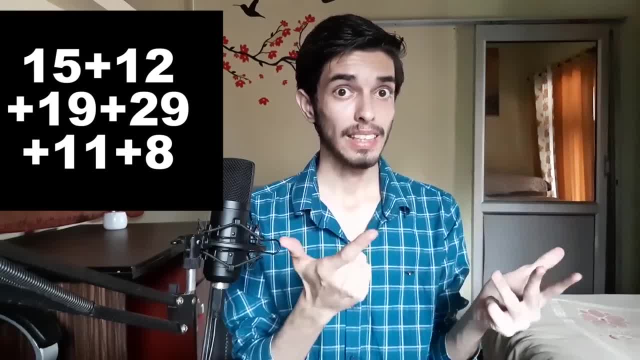 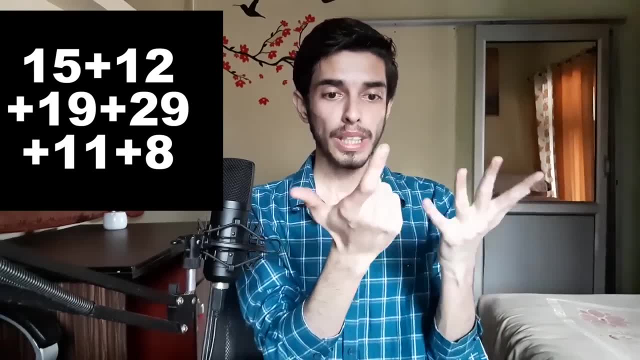 us the next number. So add 11.. 10,, 11.. Now add 8 in here. So for adding 8, we will add 10 and subtract 2.. We can't subtract 2 in here because like we don't have two fingers up, So what we can. 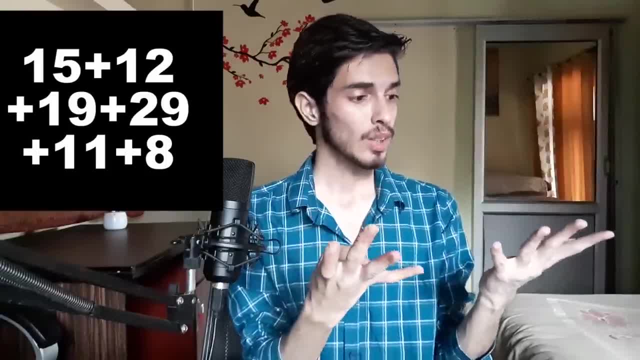 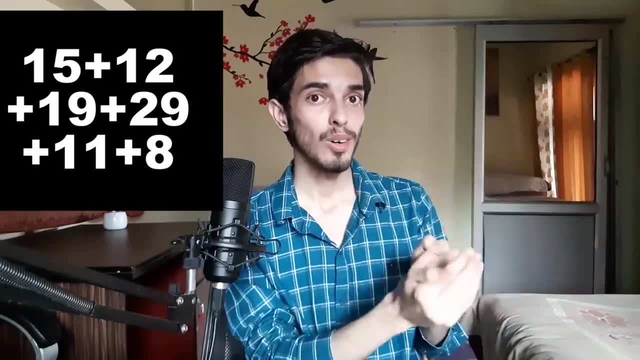 do is this: We can subtract 5 and then add 3.. So what do we have in here? We have 90 and 4.. So 94 is our answer. So this is how we use cheese and bob to do those addition kinds of. 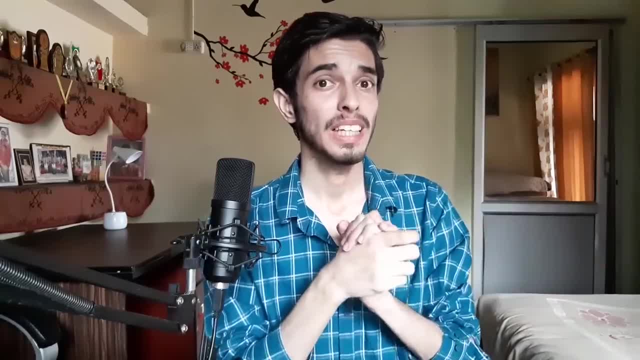 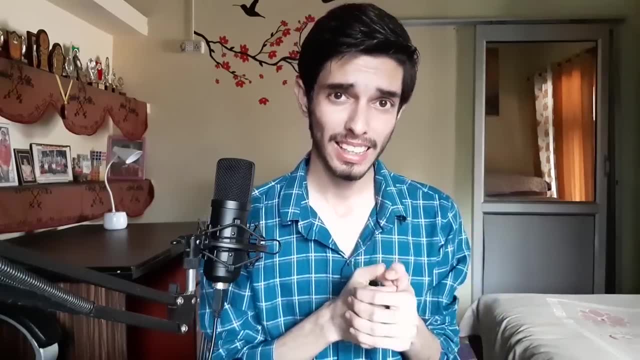 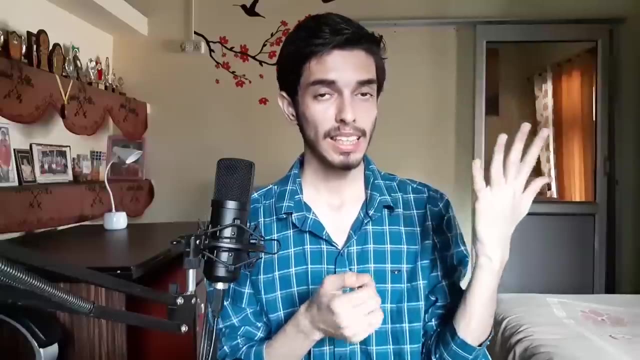 problems. Now, what you have learned is almost all the cheese and bob that you need to know. Now the only thing you need to go beyond 100 is the representation of 100. So it is pretty simple. See, this is 10, 20,, 30,, 40,, 50,, 60,, 70,, 80,, 90,, 90.. And this is 91, 92, 93, 94, 95, 96, 97,, 98, 99. 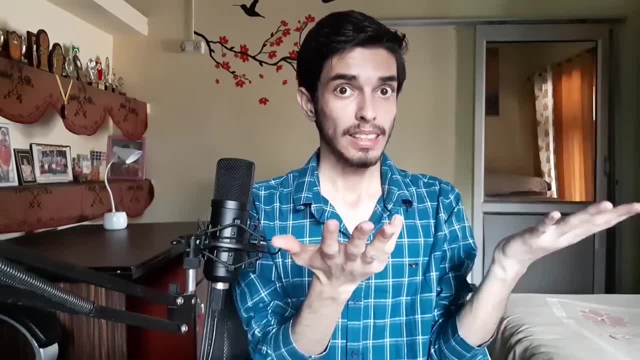 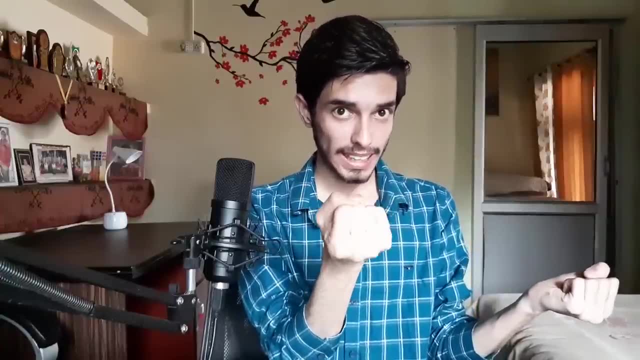 Now, if you want to represent 100, then what do we do? is this? Like we close everything, Like we are going in the next level, So closing everything And use your right hand, because it was in 99.. Now, if you like, hold your hand like this: Now, this is representing 100. And your this? 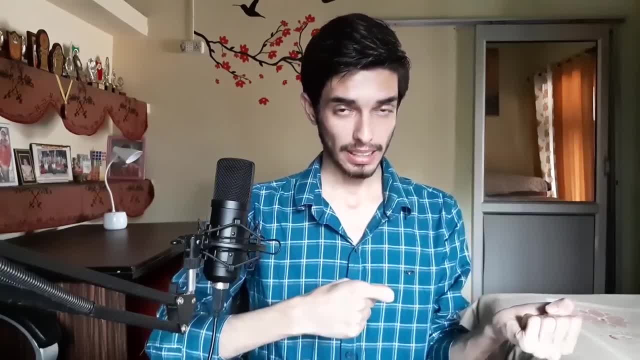 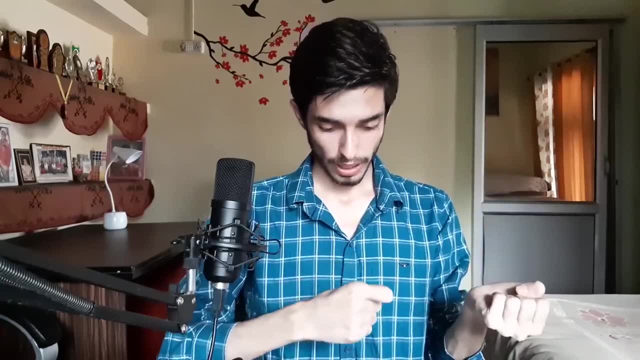 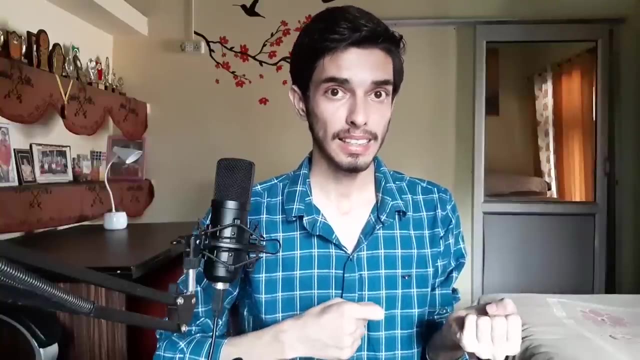 this finger should be like this. So this is for 100.. Now how you read it: You first read right, then read left and then read right. So this is basically 100.. This is 0 and this is also 0 because no other finger is open. So this is representing 100.. Now this, this is representing. 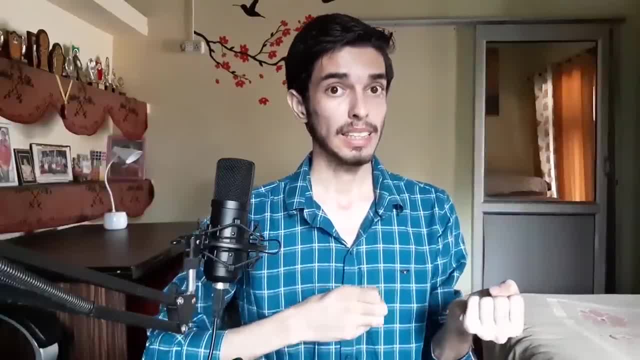 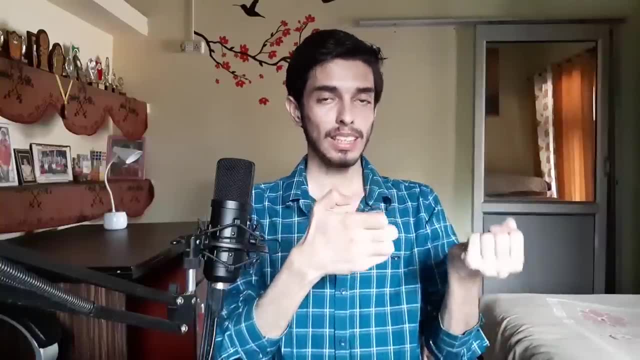 200.. This like half open. This is representing 300, 400, now 500, 600, 700, 800 and 900.. So this is basically the same thing. Just half open fingers and hand like this represent that. 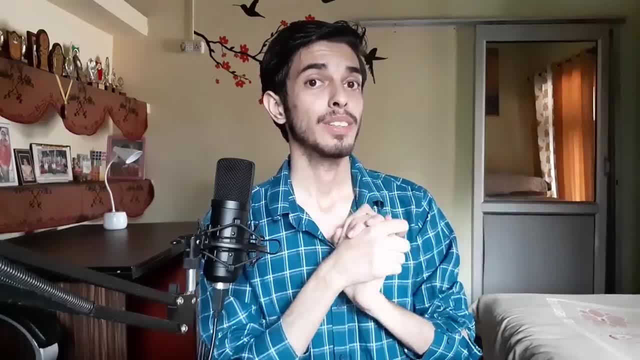 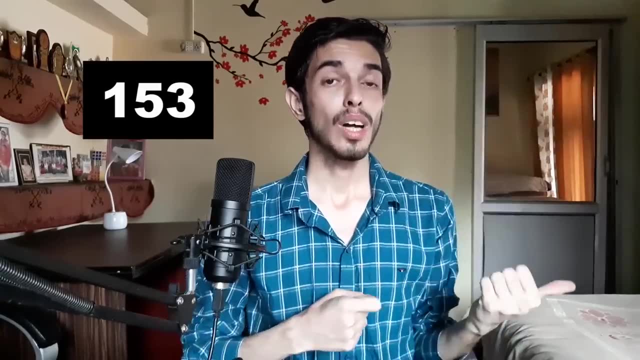 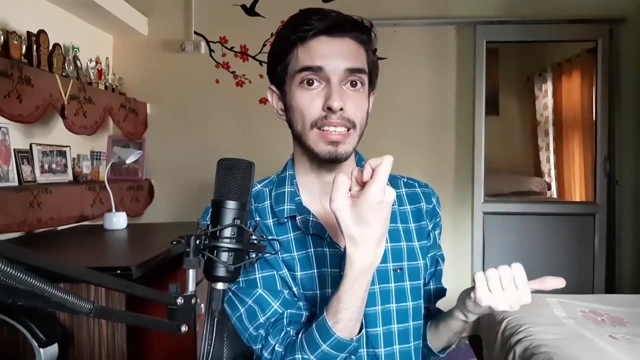 you are in hundreds. Okay, Now try representing 153 on your hands. So now let's represent 153.. So this is 100 and this is 50.. Now representing 3.. So now for representing 3, this finger is representing 100.. We also need to represent one with it. What do we do? We half open it and then 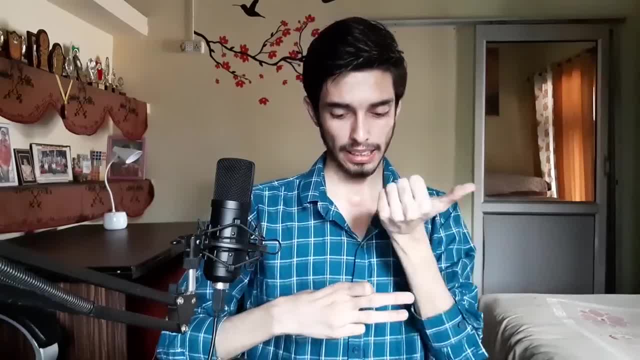 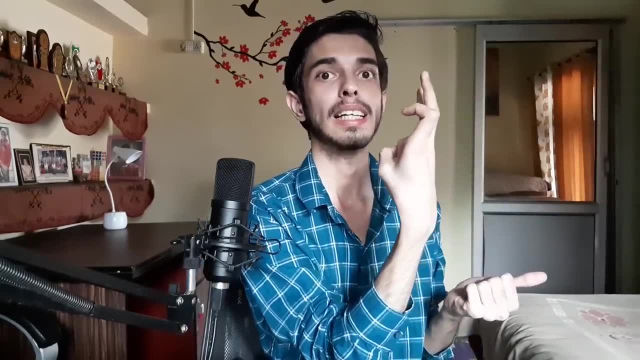 full open the other two fingers. So this is representing basically, like this: This is 100, 50 and this 3, because this is now half open. This is not like this. This is like this. So now you can see, as we are going further, our hands are getting a little bit messier. 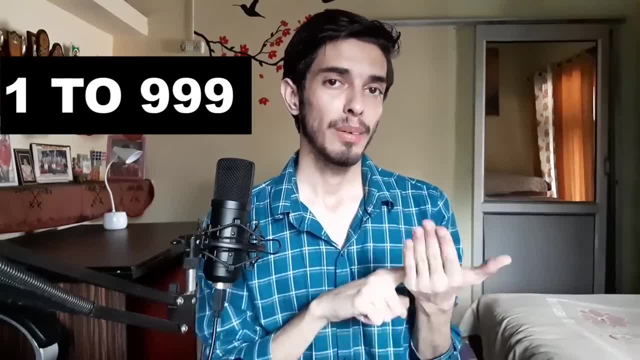 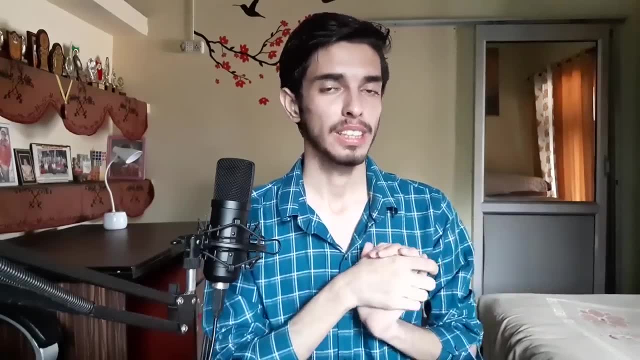 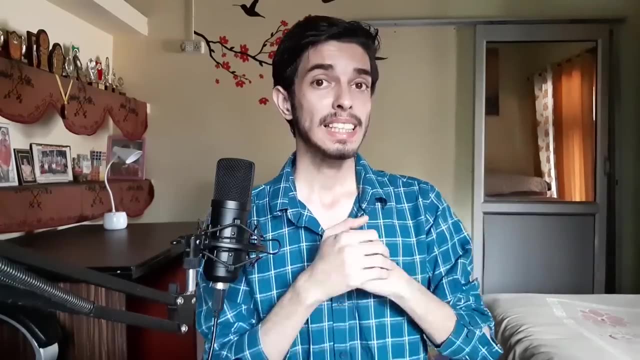 This is why I will teach you to only count till 999.. Because after that our hands get a lot, lot messier, and mathematics goes somewhere like this, and it is only Kung Fu which is left. So we will count till 999.. Now let's do a simple addition. problem with this method. So add 68 and 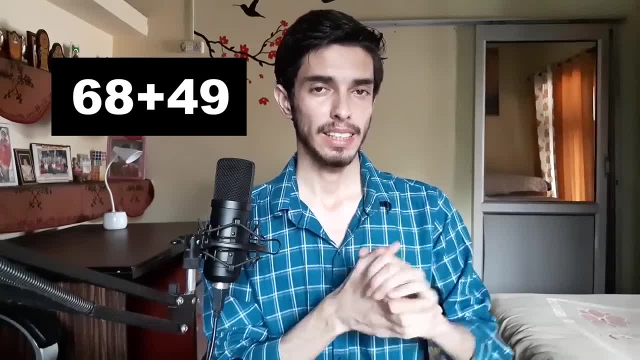 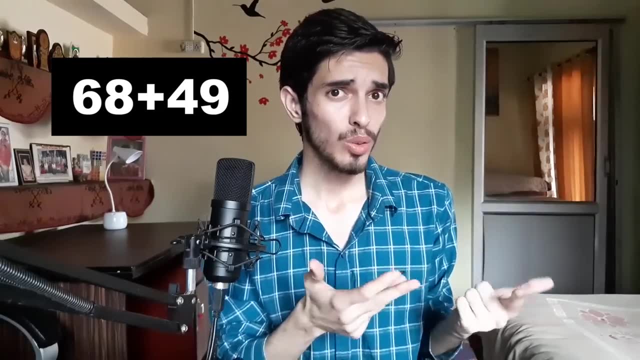 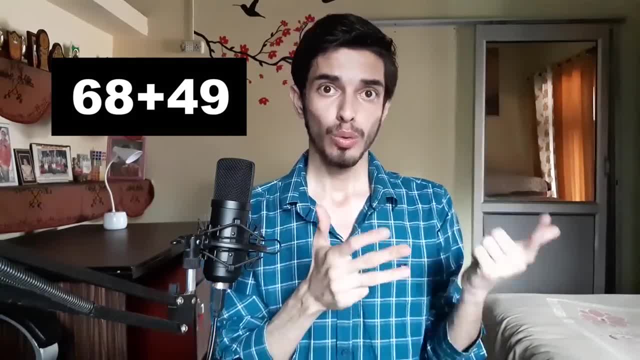 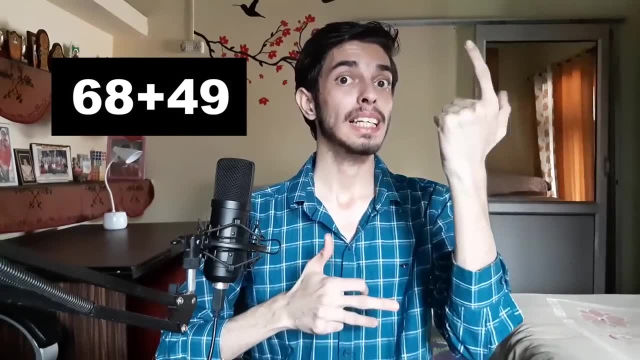 How would we do it? Because we have just three fingers left in here. So what we can do is this: We can add 100 and like, close this half 100, and then we can subtract 60. So we have added 40.. 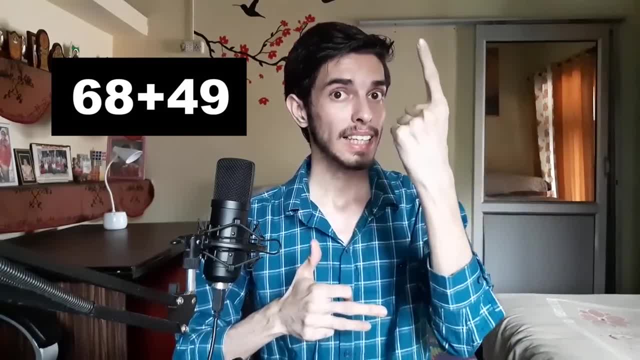 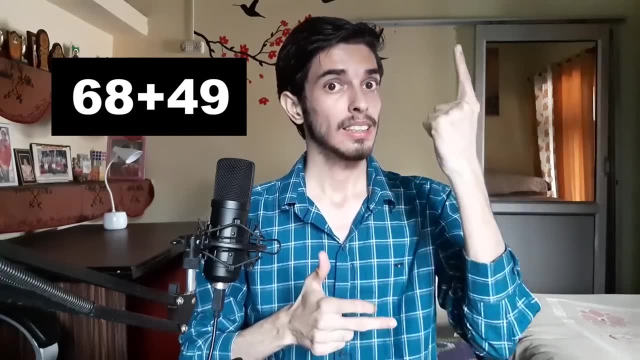 Now we need to add a 9.. For adding 9, we can like add a 10 and subtract 1, like subtracting 1 and this finger like half open. So what we have in here see 100,. this is representing 10 and this. 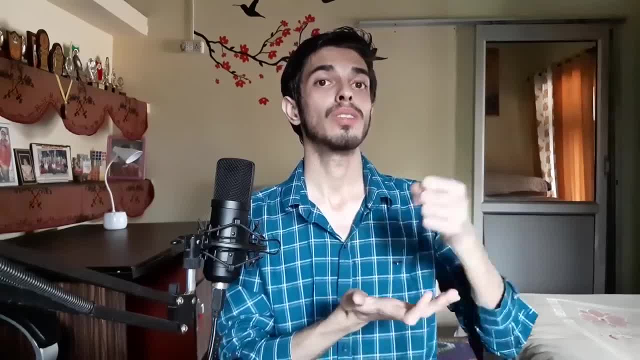 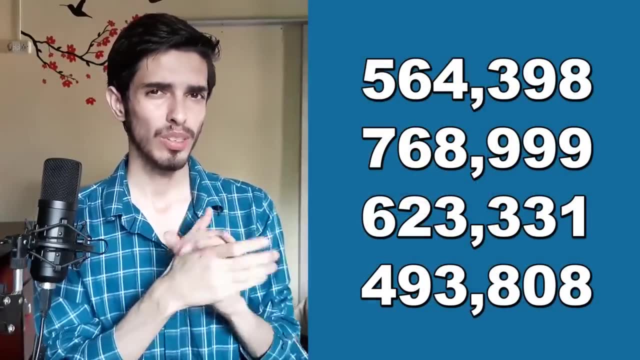 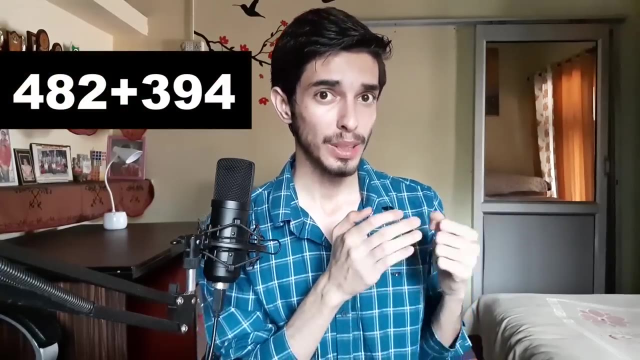 17 is our answer. So this is how, basically, we can do problems beyond 100 using Chisholm Bob. So now, finally, try representing these numbers on your hands as swiftly as you can, And if you can do it, I have a challenge for you. You can try doing this problem. Add 482 and 394 using Chisholm. 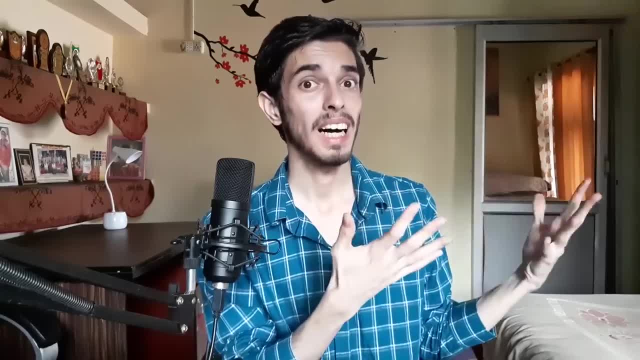 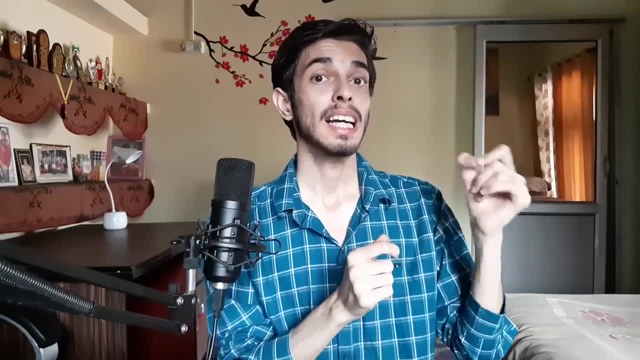 Bob, And if you can do it, then congratulations. you are a master at Chisholm Bob. So just a fact. in reality, we can represent every numbers till 9,999 on our hands. This is the power of Chisholm Bob, but I'm not teaching it. 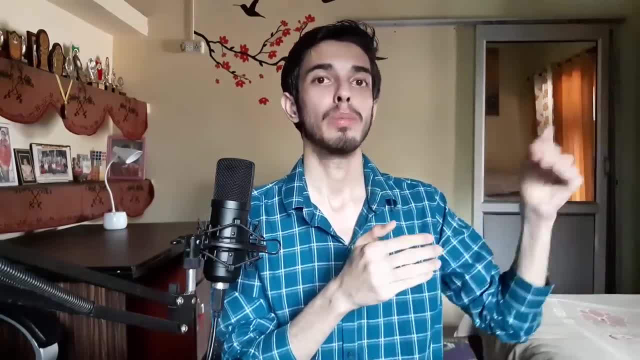 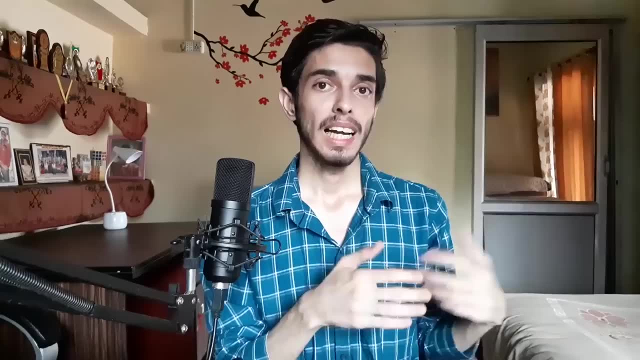 because this was already messier and that is more, more messier. But if you want to learn it, you can learn it from this book And, as I always say, you need to practice it. And if you watch my previous video, I have said it many times: for practicing, I have made a game known as Math. 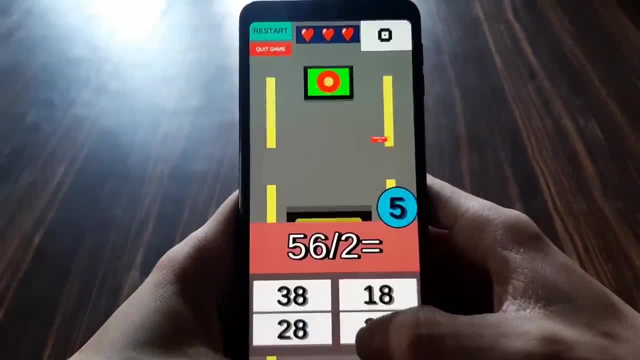 Blob Run, in which there is a good blob and bad blob. The bad blob wants to eat our good blob, but solve the problem. So if you want to learn it, you can learn it from this book And if you have any questions regarding mental math questions, we'll save your blob So you can use that game to. 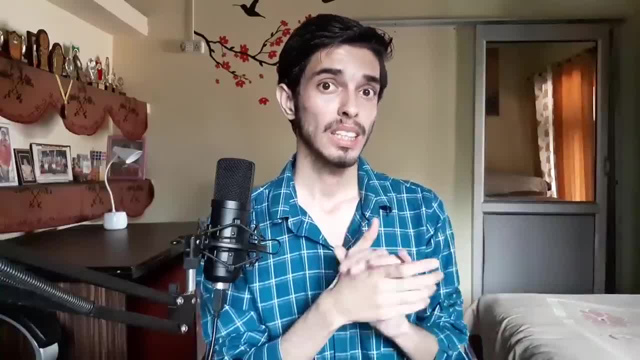 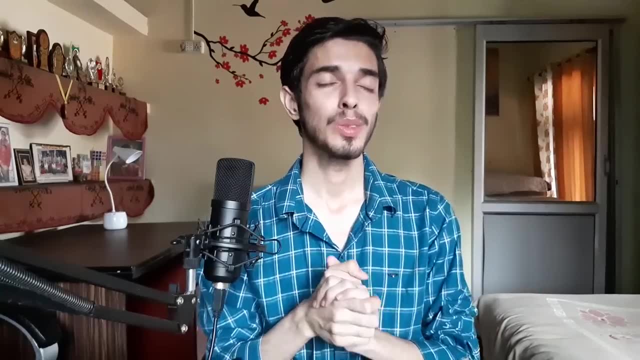 practice Chisholm Bob too, And also do not forget to join us on our Discord server. There we are making a really good maths community. And finally, thanks for watching this video. I hope you have enjoyed and always remember that math is everything.